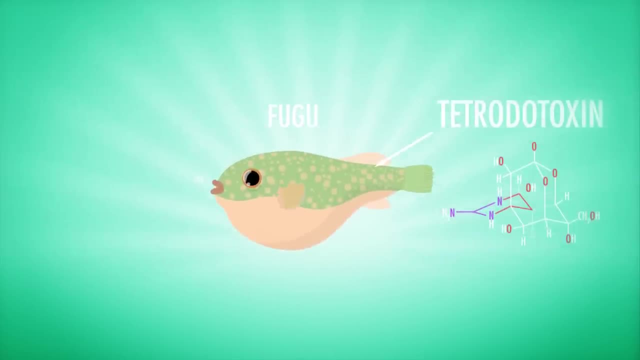 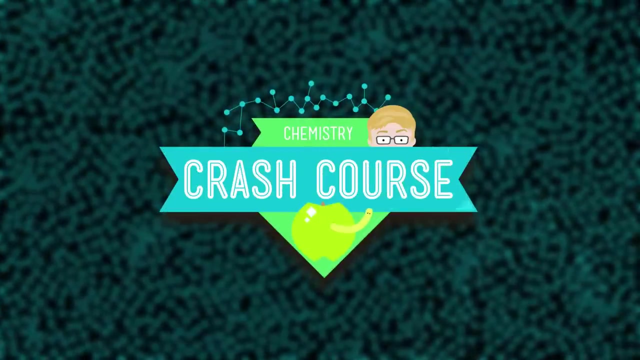 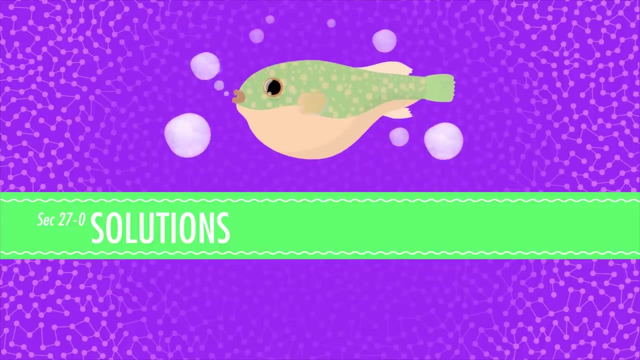 the bubbles in Coca-Cola or the toxin in the tissues of the Japanese pufferfish. what usually matters most about a solution is how much solute is in it. Often in the lab we use placeholders like dilute and concentrated. when we're doing, 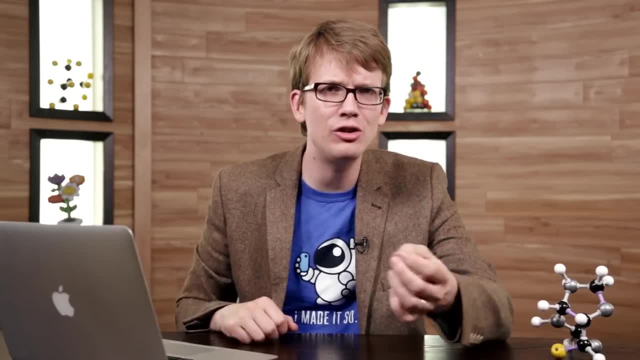 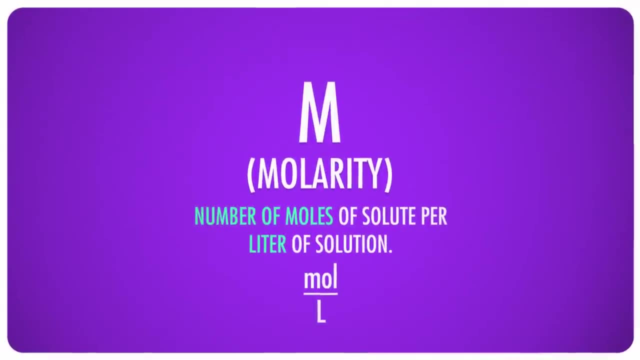 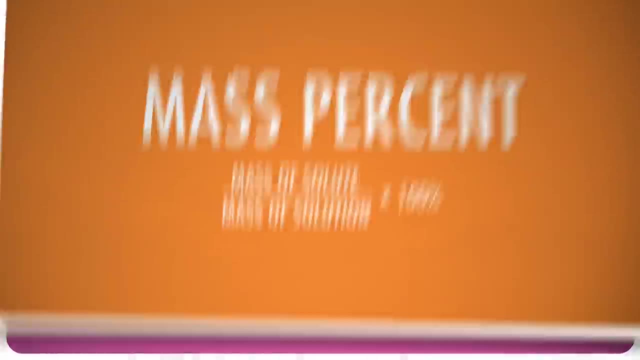 a solution. But those are vague terms and we should generally be as precise as possible. Here are a few ways to do that. We can describe a solution by its molarity: the number of moles of solute per liter of solution. its molality- the number of moles of solute per kilogram of solvent or its 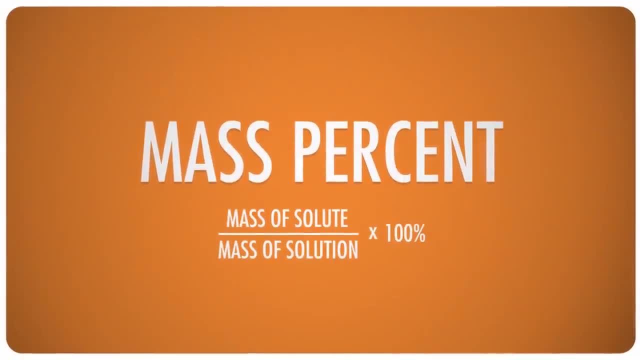 mass percent. The mass percent of a solution is the mass of the solute divided by the mass of the solution all multiplied by 100. So in a can of your average soft drink there's about 33 grams of sugar and a total mass of 350 grams. that's half of the solute you're 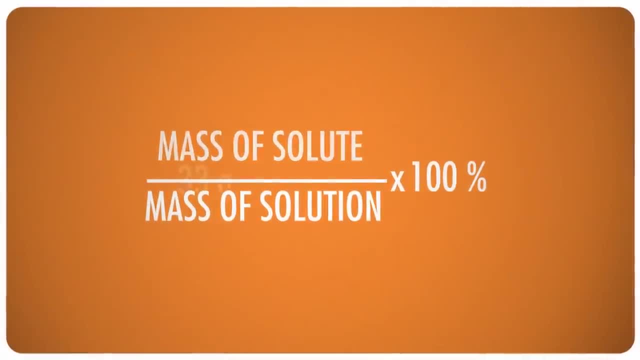 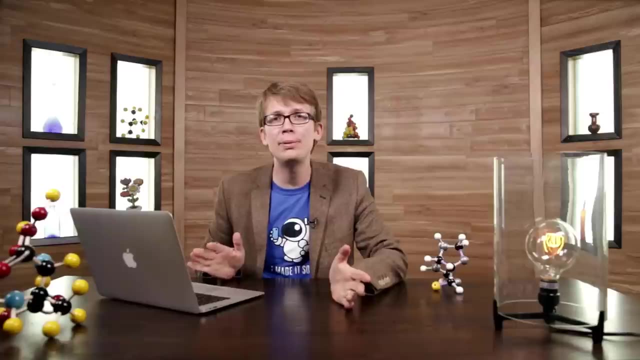 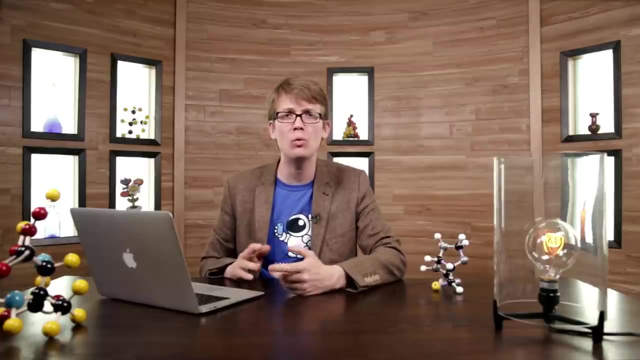 using 55 grams. Divide the mass of the solute by the mass of the whole thing, times 100, and the mass percent of the sugar in solution is 9.2%. Easy peasy there. but the more interesting question here is why. Why can you even dissolve so much sugar in a can of soda? And what about? 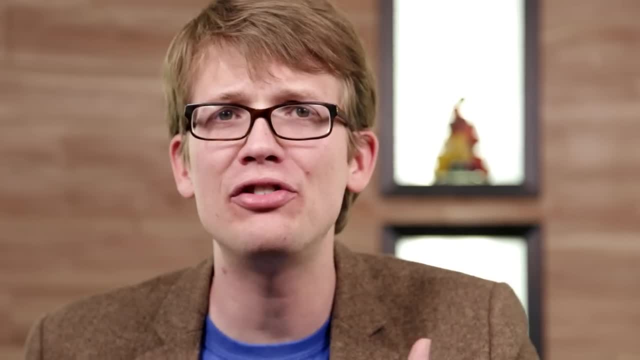 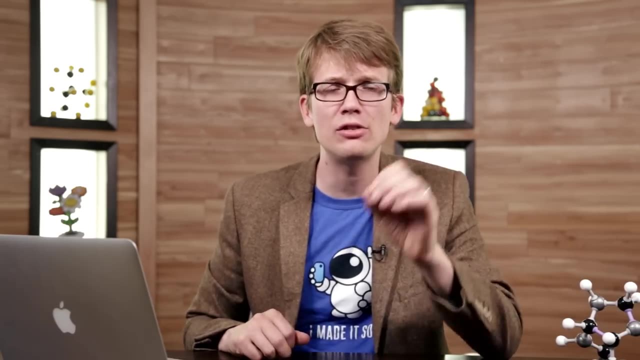 all that carbon dioxide gas. What's happening here? How does the stuff go in the stuff and where does it go? And what's actually happening at the molecular level? Well, the first thing to keep in mind is that not every solvent can dissolve every solute. Gas molecules don't interact that strongly, so gases pretty much always dissolve in each other. But liquid solvents have a ton of molecular interaction, so the structure of the individual molecules determines whether a substance will dissolve and how well it will dissolve- Polarity. 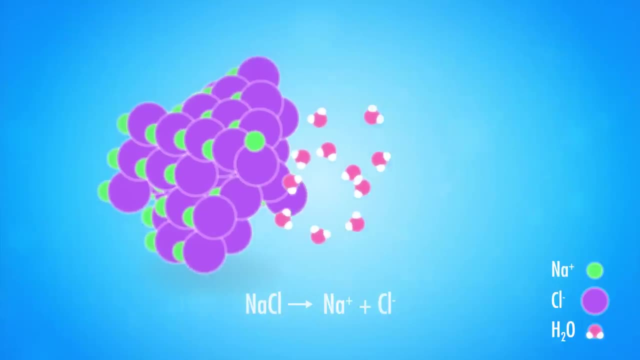 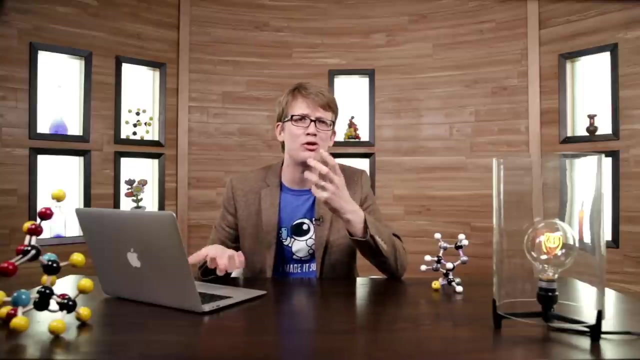 is, of course, the biggest bit of this. For a substance to dissolve, it needs to interact favorably with the solvent. This only happens if they have similar polarities, which allows them to form cool in-solution structures, spacing the solute particles out evenly. 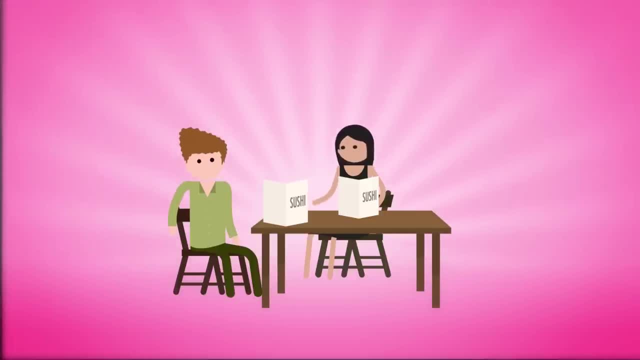 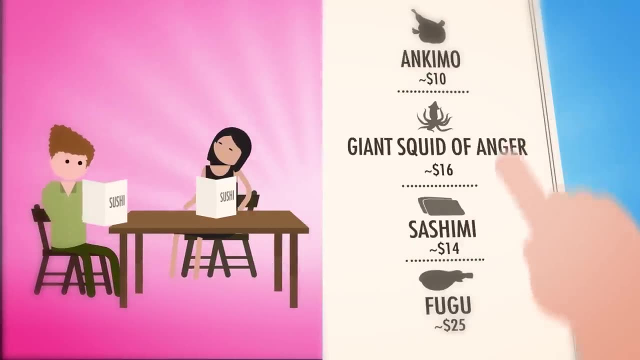 Topic change. Say you're on a first date at a sushi restaurant and you want to be all cool and nonchalant and I'll tangle with death if death wants me to. so you order the puffer fish, otherwise known as fugu. Fugu contains a poison called 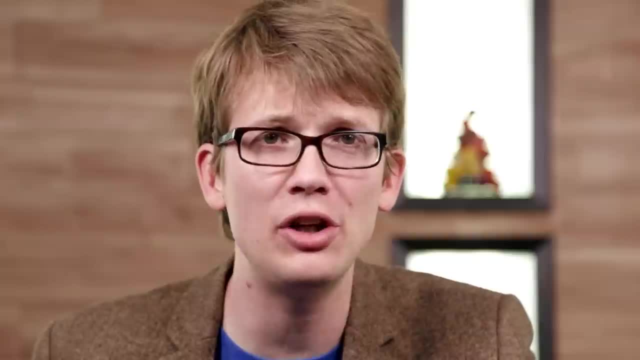 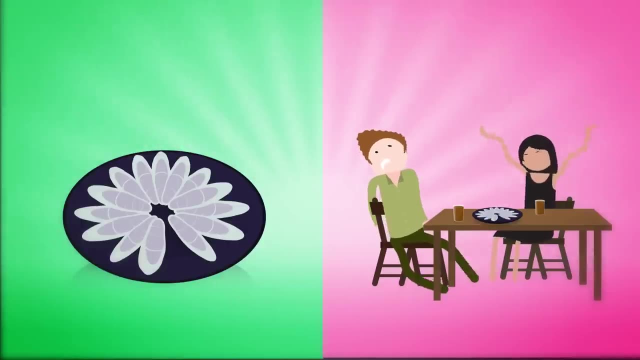 tetrodotoxin, and even in the hands of chefs who know what they're doing. it makes your lips go numb just at the taste of it. If the chef makes a mistake and you eat the wrong part of the fish, the tetrodotoxin will mess with your nervous system and cause paralysis. 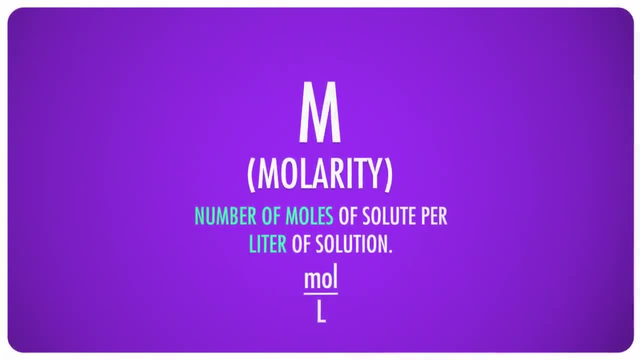 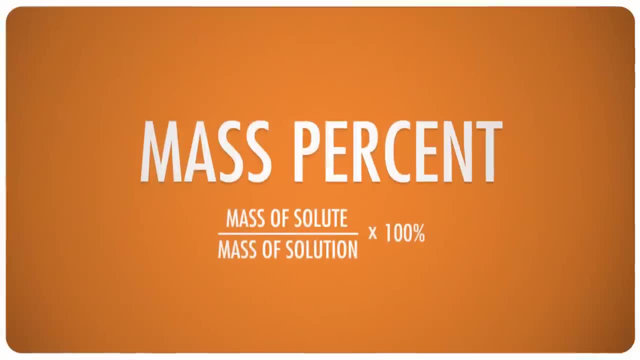 We can describe a solution by its malarity- the number of moles of solute per liter of solution, Its malality- the number of moles of solute per kilogram of solvent, Or its mass percent. The mass percent of a solution is the mass of the solute divided by the mass. 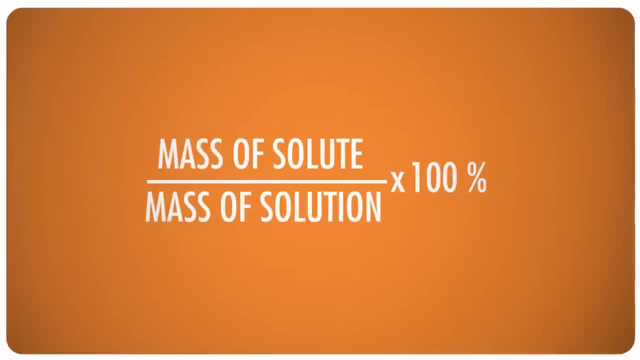 of the solution all multiplied by 100. So in a can of your average soft drink with about 33 grams of sugar and a total mass of 350 grams of sugar, you can measure the volume of a solution as the mass of the solution And that's the number of moles of solute per. 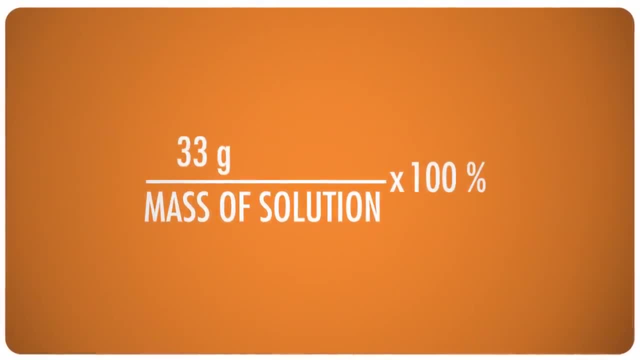 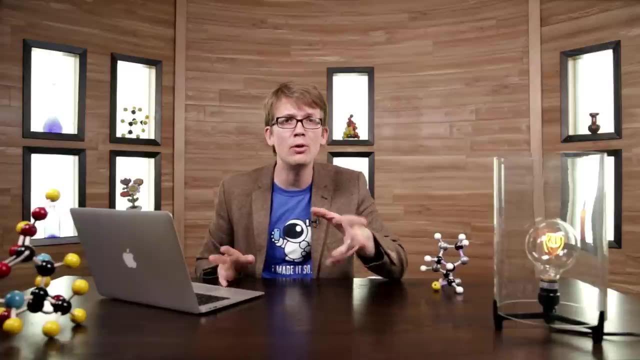 mass of 355 grams. Divide the mass of the solute by the mass of the whole thing, times 100, and the mass percent of the sugar in solution is 9.2%. Easy peasy there. but the more interesting question here is why. Why can you even dissolve so much sugar in a can of soda? And what about? 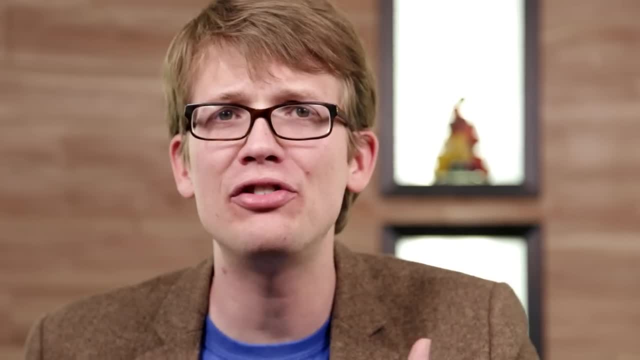 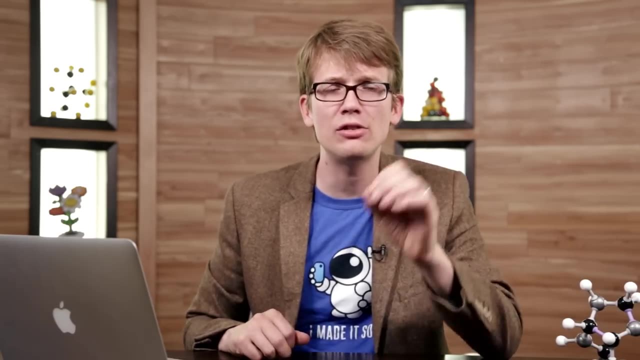 all that carbon dioxide gas. What's happening here? How does the stuff go in the stuff and where does it go? And what's actually happening at the molecular level? Well, the first thing to keep in mind is that not every solvent can dissolve every solute. Gas molecules don't interact that strongly, so gases pretty much always dissolve in each other. But liquid solvents have a ton of molecular interaction, so the structure of the individual molecules determines whether a substance will dissolve and how well it will dissolve- Polarity. 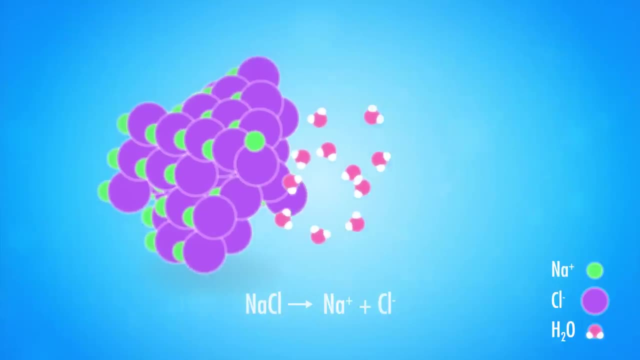 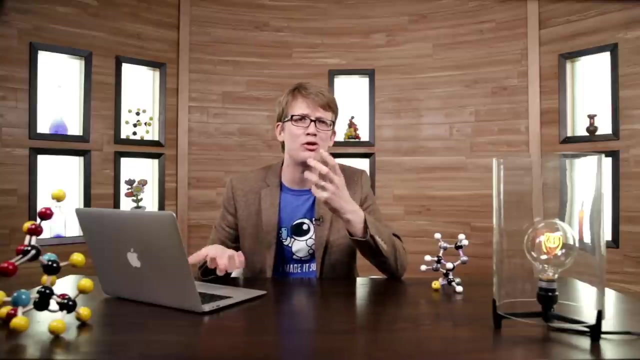 is, of course, the biggest bit of this. For a substance to dissolve, it needs to interact favorably with the solvent. This only happens if they have similar polarities, which allows them to form cool in-solution structures, spacing the solute particles out evenly. 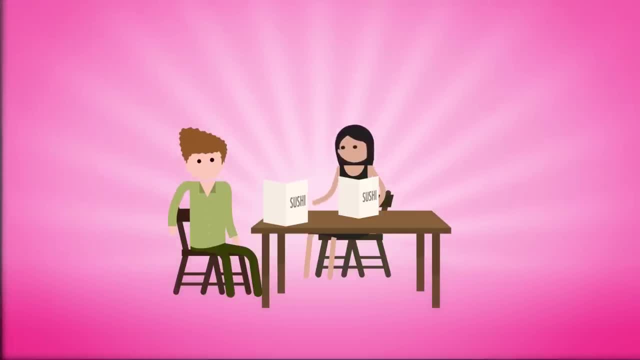 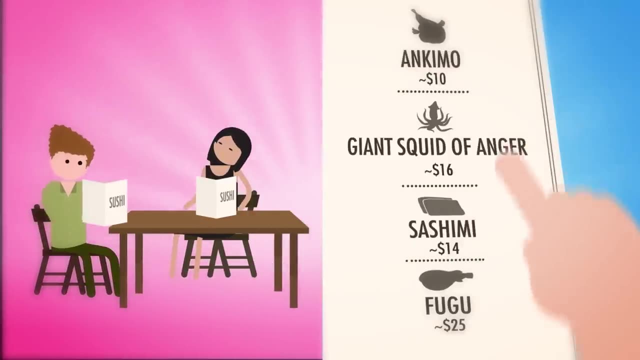 Topic change. Say you're on a first date at a sushi restaurant and you want to be all cool and nonchalant and I'll tangle with death if death wants me to. so you order the pufferfish, otherwise known as fugu. Fugu contains a poison called tetrodotoxin, and even in the hands of chefs who know what they're doing. it makes your lips go numb just at the taste of it. If the chef makes a mistake and you eat the wrong part of the fish, the tetrodotoxin will mess with your nervous system and cause paralysis. 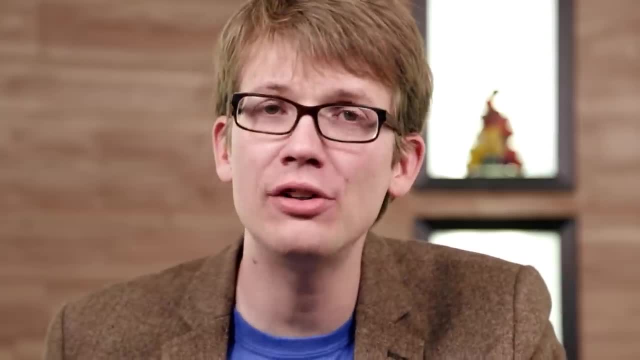 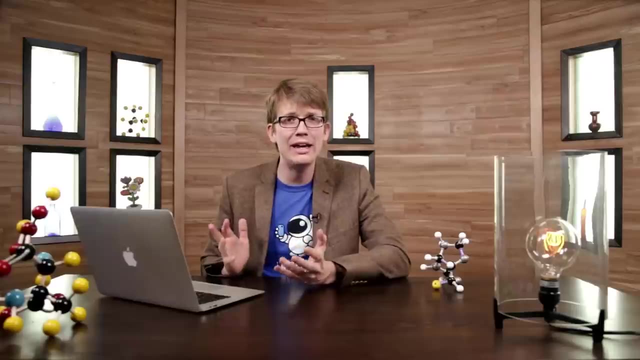 suffocation, maybe some death. Why? Well, in part because of its polarity And yours. Tetrodotoxin is covered on its outer surface with polar alcohol and amine groups, so it dissolves easily in polar solvents like water, And who's made mostly of water. So if you've watched Crash Course Biology, 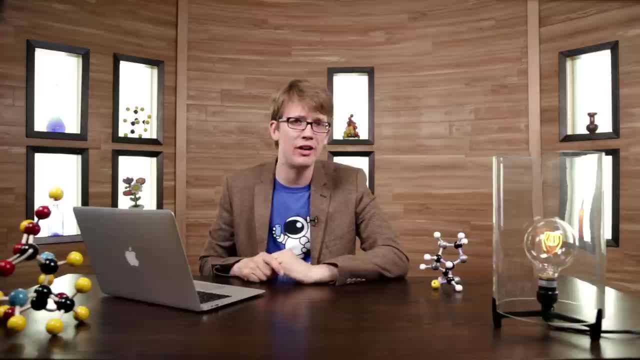 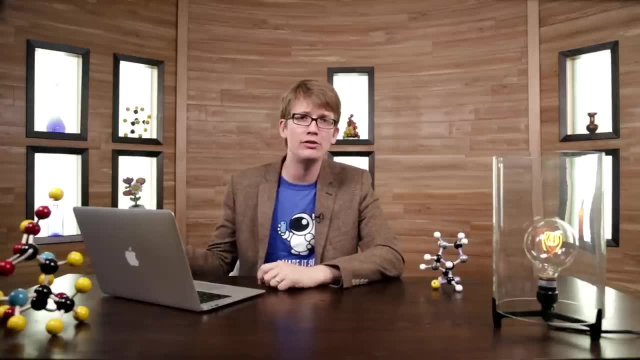 you know all about sodium channels, the tunnels on the outside of nerve cells that allow them to communicate with each other. Well, tetrodotoxin is really good at binding to those channels, messing up your nervous system and killing you, Because it's so polar, and your body. 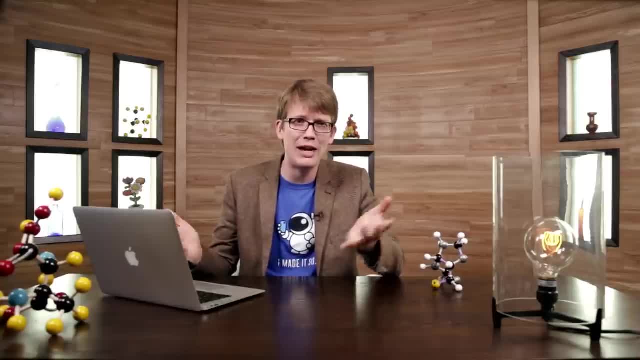 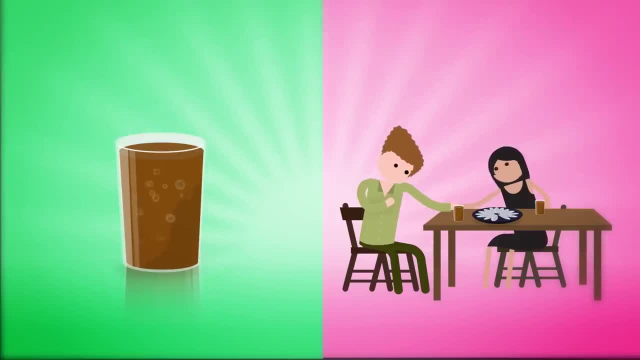 is just one big aqueous solution. tetrodotoxin pretty much has free rein to just jump on every sodium pump. you got On to the next attribute that affects solubility. Let's assume that you've survived the first course of your meal and you order a soda pop To get all those little bubbles that make. 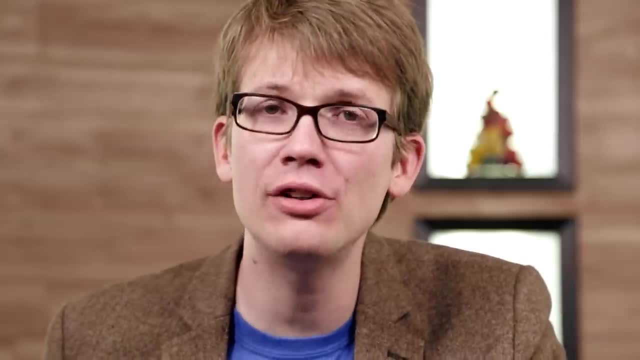 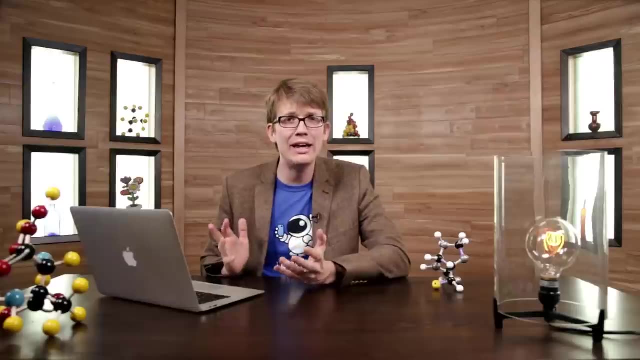 suffocation, maybe some death. Why? Well, in part because of its polarity And yours. Tetrodotoxin is on the inside or surface, with polar alcohol and amine groups, so it dissolves easily in polar solvents like water, And who's made mostly of water? 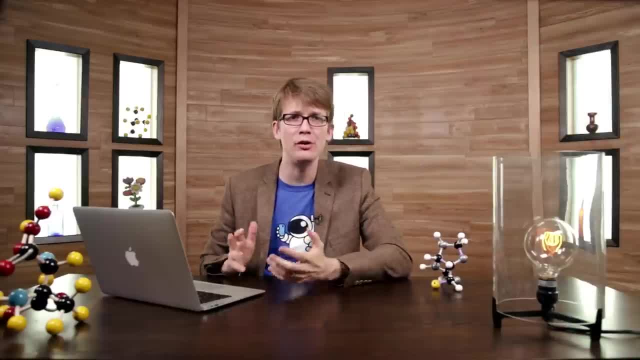 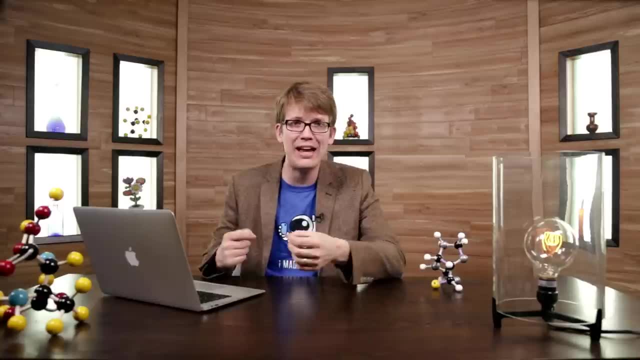 So if you've watched Crash Course Biology, you know all about sodium channels, the tunnels on the outside of nerve cells that allow them to communicate with each other. Well, tetrodotoxin is really good at binding to those channels, messing up your nervous system and killing. 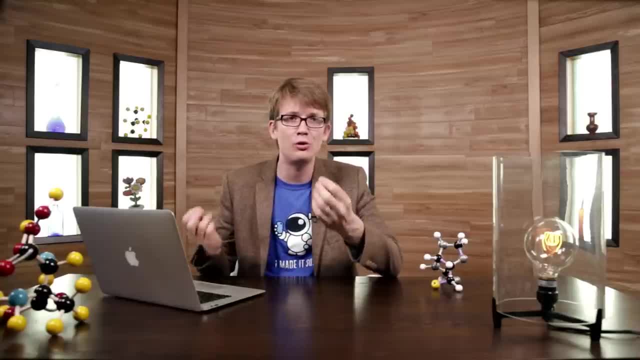 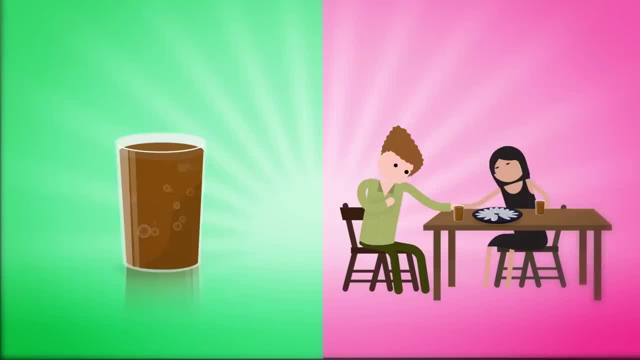 you Because it's so polar and your body is just one big aqueous solution. tetrodotoxin pretty much has free rein to just jump on every sodium pump. you got On to the next attribute that affects solubility. Let's assume that you've survived the first. 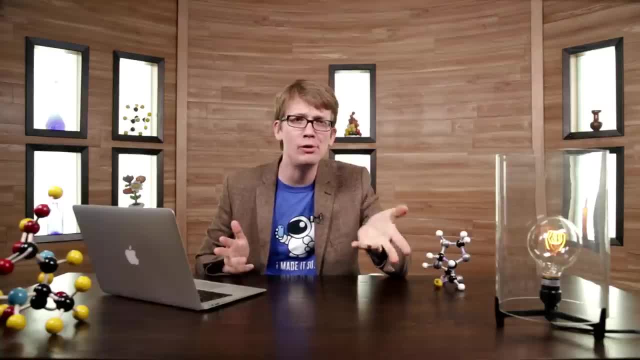 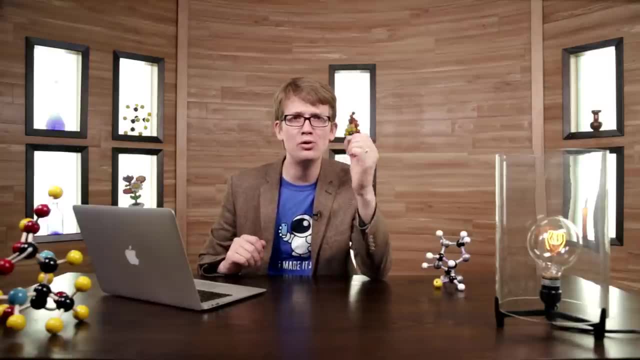 course of your meal and you order a soda pop To get all those little bubbles that make carbonated beverages so refreshing and dingly. carbon dioxide must be dissolved in the water. But how do you shove a gas into a liquid? A gas gets dissolved into a solution, the same. 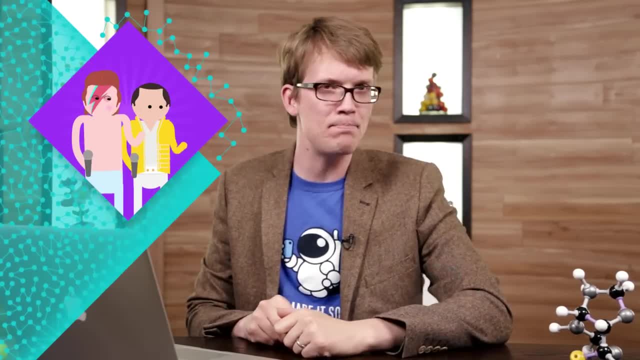 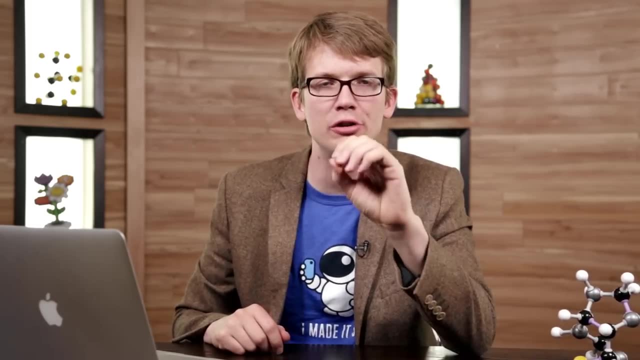 way David Bowie and Freddie Mercury collaborate Under pressure. What, As previously noted, I am old. It's not just the pressure outside of the solvent, it's the partial pressure of the solute. Partial pressure is the portion of pressure caused by the gas we're interested in In 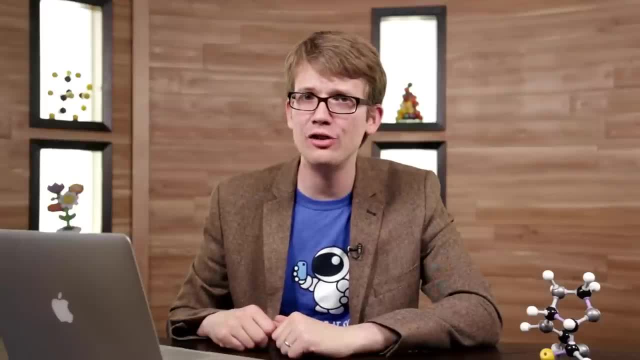 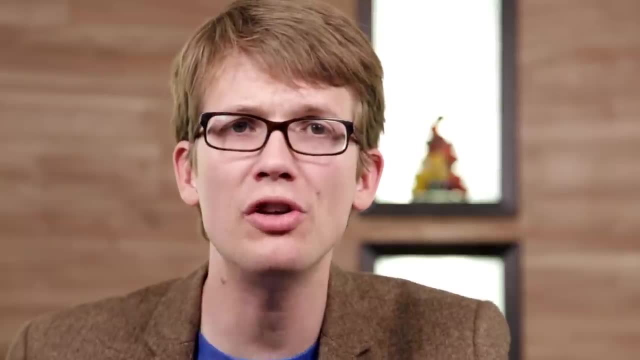 this case carbon dioxide Gas molecules, as long as they have kinetic energy, are going to want to escape the solution, so they will be creating an upward pressure on the surrounding gas In order to keep the CO2 dissolved. the partial pressure of carbon dioxide in the gas outside the solution has to be equal to or higher than the pressure of the carbon dioxide molecules pushing their way out of the solution. That's why soda bottles are nice and taut when you squeeze them. That little bit of gas up there is pressurized. 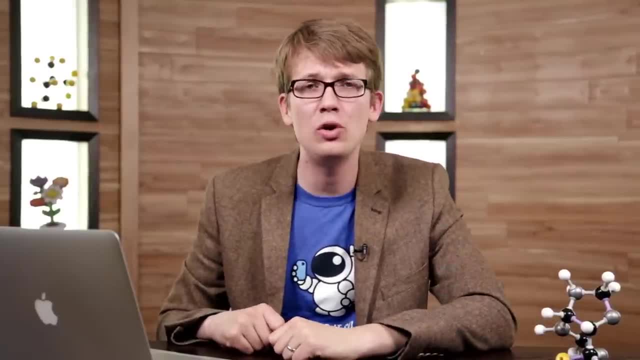 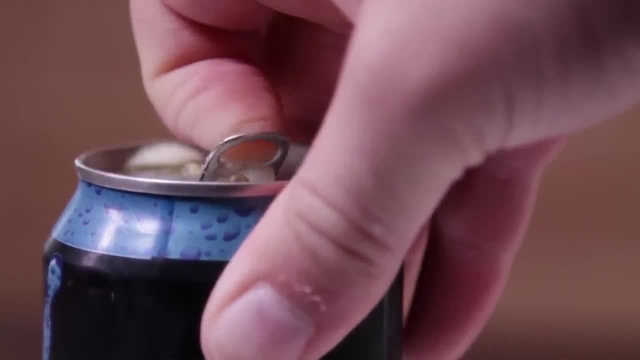 carbon dioxide And also why, when you open the can, a huge rush of carbon dioxide molecules bubble out of the soda. because the normal partial pressure of CO2 in the atmosphere isn't enough to keep it from escaping. So to get the carbon dioxide in there, all you need to do is dramatically increase the. 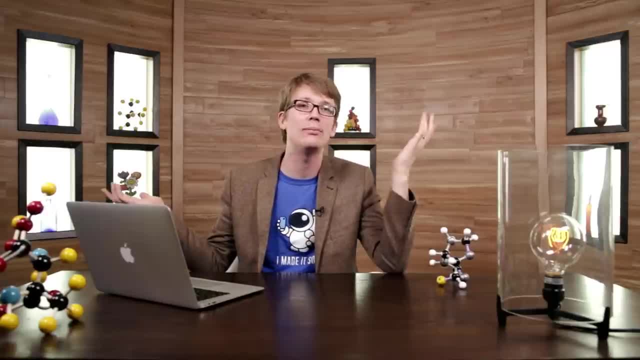 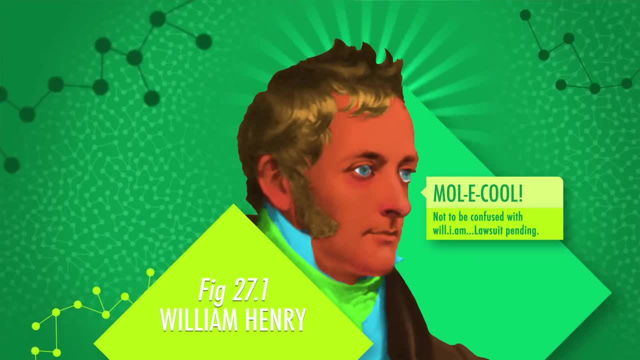 pressure of CO2 outside the liquid, And this is what's done in soda manufacturing plants. In fact, if you have a soda stream, you can do it right in your own home. Now it's easy to calculate this change in pressure, thanks to William Henry, a friend. 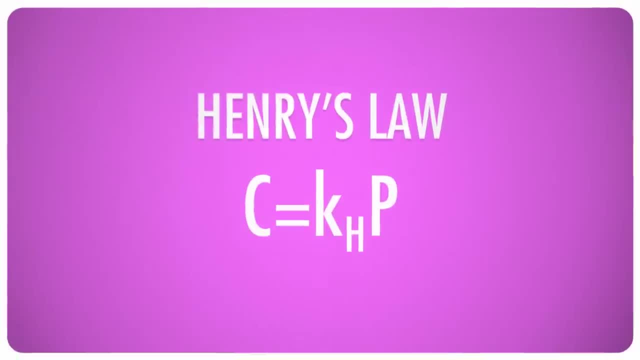 of John Dalton of Dalton's Law of Partial Pressures. According to Henry's law, the concentration of a dissolved gas equals the partial pressure of the gas above the solution multiplied by a constant that expresses the solubility of the gas in that solution. 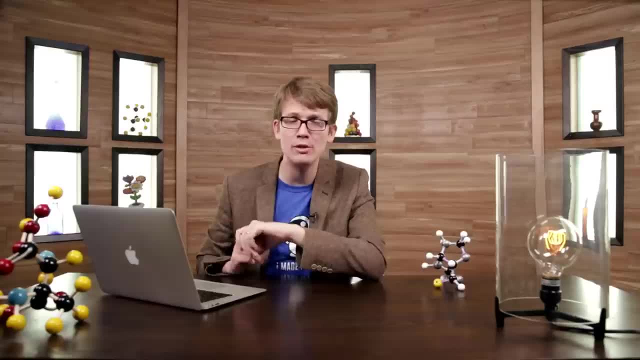 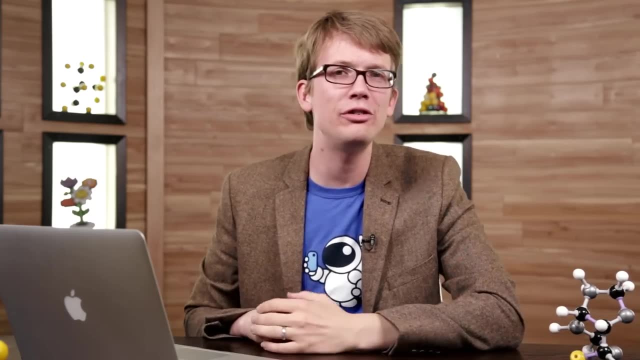 carbonated beverages, so refreshing and dingly. carbon dioxide must be dissolved in the water. But how do you shove a gas into a liquid? A gas gets dissolved into a solution. the same way, David Bowie and Freddie Mercury collaborate Under pressure. What, As previously noted, I am old. It's not just the pressure outside of the solvent, it's the partial pressure of the solute. Quick review: Partial pressure is the portion of pressure caused by the gas we're interested in, In this case carbon dioxide Gas molecules, as long as they have kinetic energy, are going. 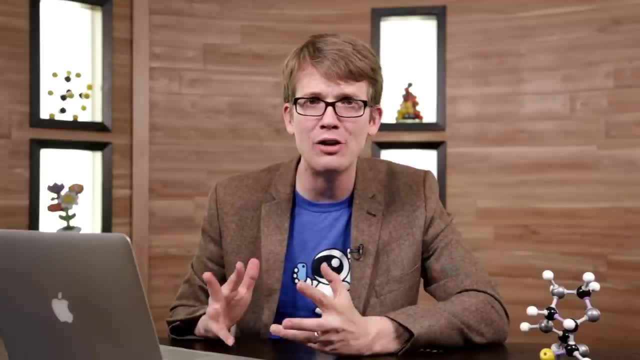 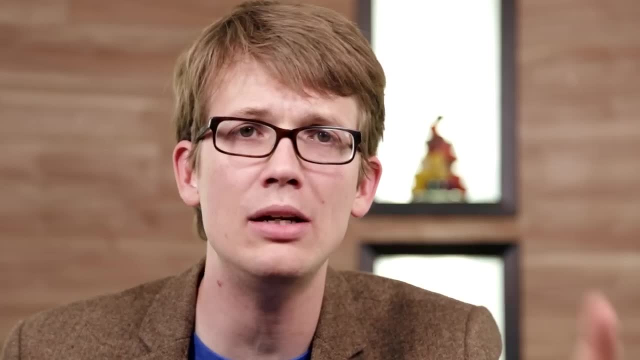 to want to escape the solution, so they will be creating an upward pressure on the surrounding gas. In order to keep the CO2 dissolved, the partial pressure of carbon dioxide in the gas outside the solution has to be equal to or higher than the pressure of the carbon. dioxide molecules pushing their way out of the solution. That's why soda bottles are nice and taut. when you squeeze them That little bit of gas up, there is pressurized carbon dioxide. And also why, when you open the can, a huge rush of carbon dioxide molecules bubble out. 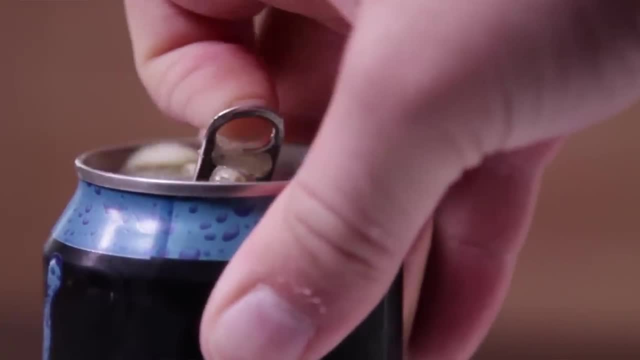 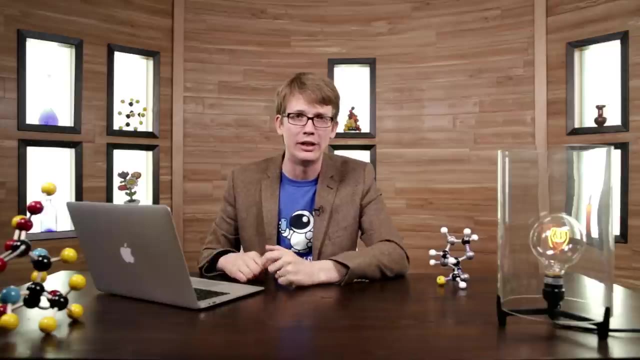 of the soda, because the normal partial pressure of CO2 in the atmosphere isn't enough to keep it from escaping. So to get the carbon dioxide in there, all you need to do is dramatically increase the pressure of CO2 outside the liquid, And this is what's done in soda manufacturing plants. 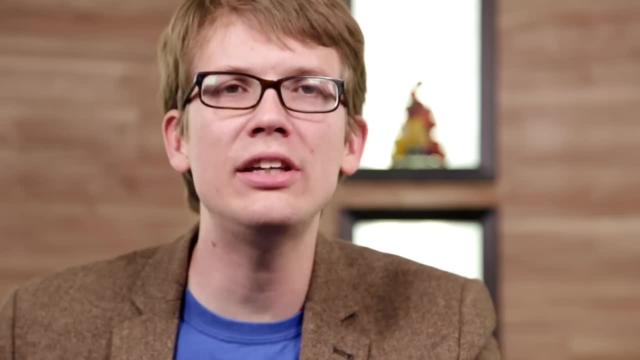 In fact, if you have a soda stream, you can do it right in your own home. Now it's easy to calculate this change in pressure, thanks to William Henry, a friend of John Dalton, of Dalton's Law of Partial Pressures. According to Henry's law, the constant pressure of CO2 is equal to the pressure of CO2 in the liquid. So if you have a soda stream, you can do it right in your own home. Now it's easy to calculate this change in pressure. so this is what's done in soda manufacturing plants. 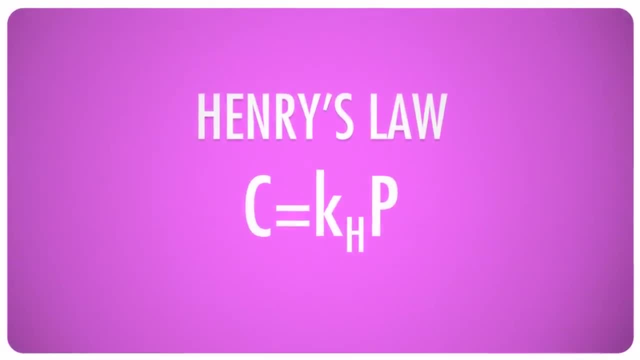 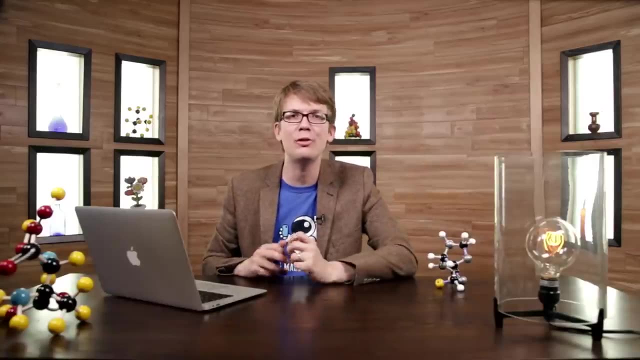 So let's make this a real problem. The concentration of a dissolved gas equals the partial pressure of the gas above the solution multiplied by a constant that expresses the solubility of the gas in that solution, And we can use Henry's Law to figure out how much carbon dioxide is dissolved in our 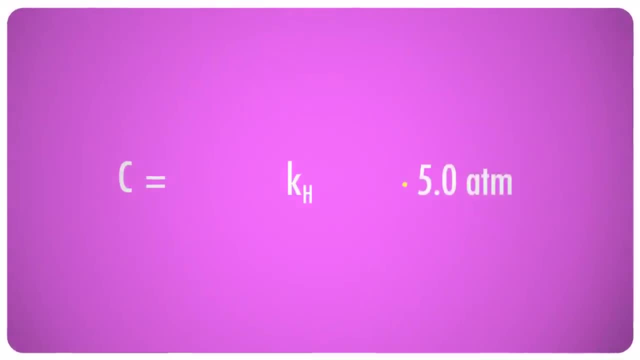 can of soda. The pressure of CO2 in a can is 5.0 atmospheres And you can look up the solubility of CO2 in an aqueous solution 3.4 times 10 to the negative 2 moles per liter atmosphere. 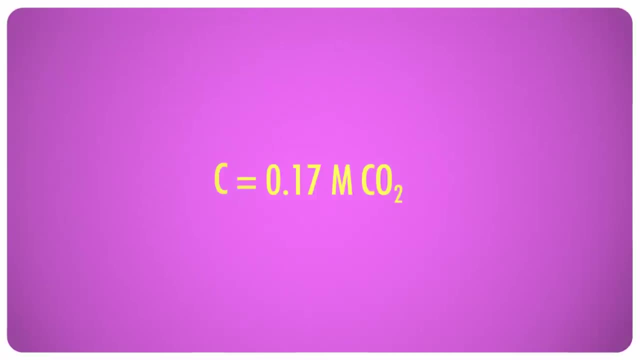 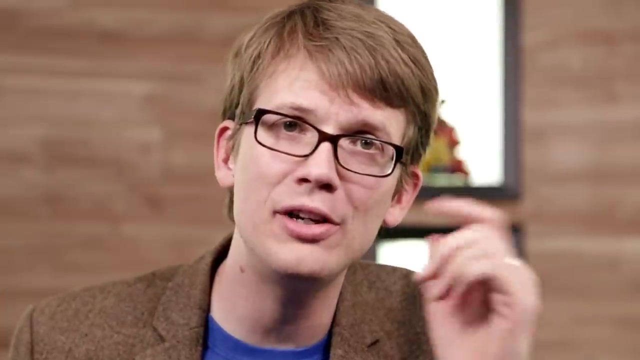 So the concentration of dissolved CO2 is 0.17 moles per liter. There are 355 milliliters or 0.355 liters of cola in a can. How much volume would that CO2 take up at normal atmospheric conditions? 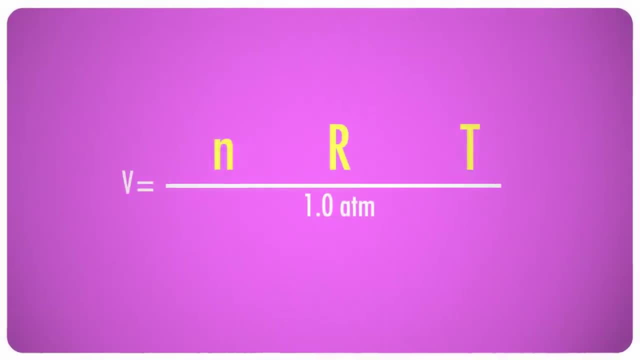 Whip out your trusty ideal gas law and we find, at atmospheric pressure and 298 kelvins or room temperature, 0.060 moles of carbon dioxide will expand to about one and a half liters. That's a lot of burps. 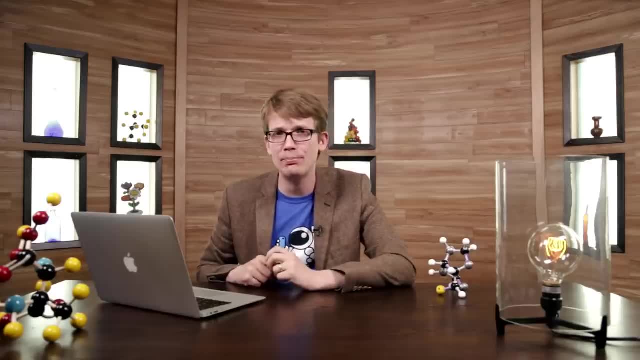 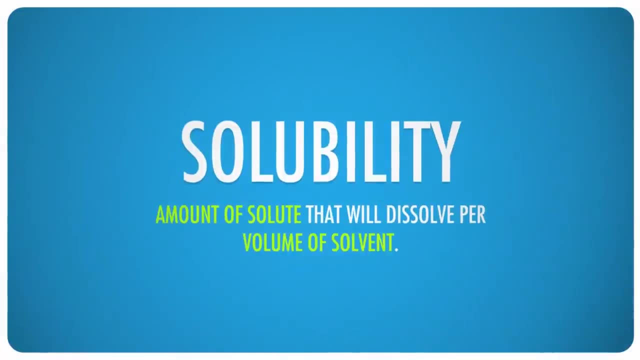 Something else to keep in mind on date night. Finally, in addition to polarity and pressure, it's temperature that affects solubility in the most complicated and therefore interesting ways. When we're dealing with solid solutes and liquid solvents, their total solubility generally. 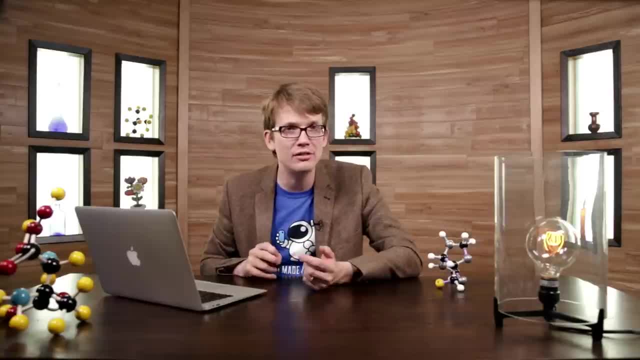 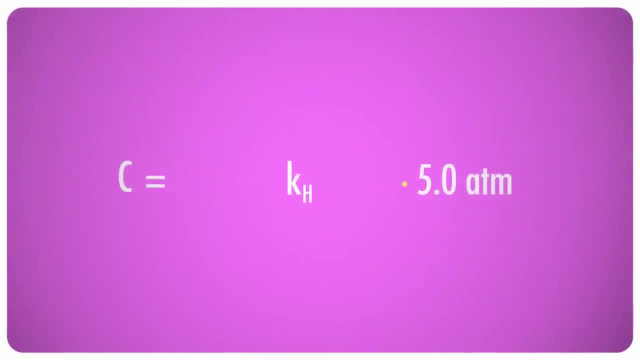 And we can use Henry's law to figure out how much carbon dioxide is dissolved in our can of soda. The pressure of CO2 in a can is 5.0 atmospheres and you can look up the solubility of CO2 in an aqueous solution 3.4 times 10 to the negative 2 moles per liter atmosphere. 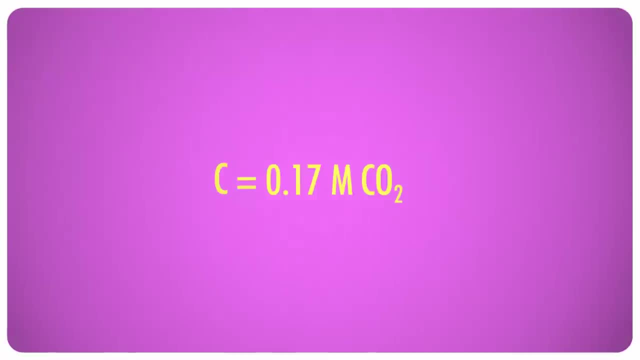 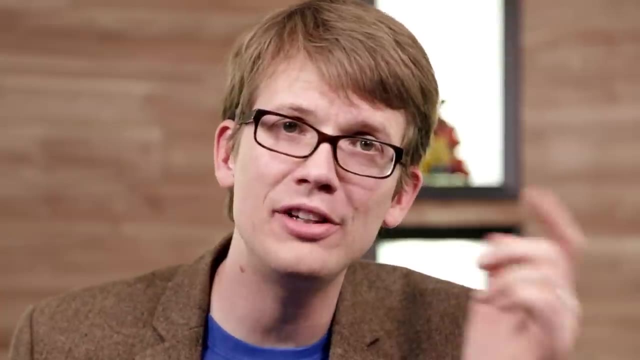 So the concentration of dissolved CO2 is 0.17 moles per liter. Now there are 355 milliliters, or 0.355 liters, of cola in a can. How much volume would that CO2 take up at normal atmospheric conditions? Whip out your trusty ideal gas law and we. 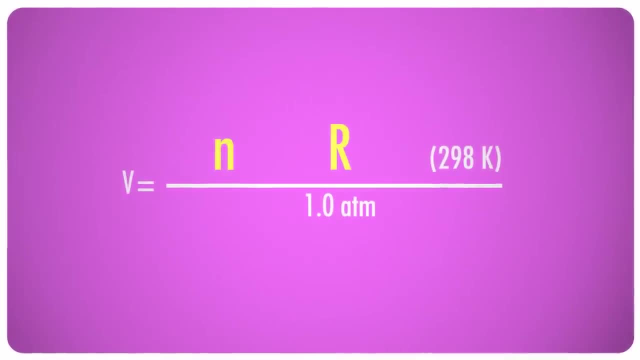 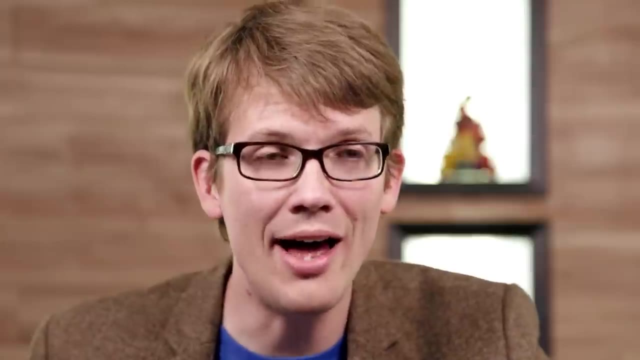 find, at atmospheric pressure and 298 kelvins or room temperature, 0.060 moles of carbon dioxide will expand to about one and a half liters. That's a lot of burps. Something else to keep in mind on date night. 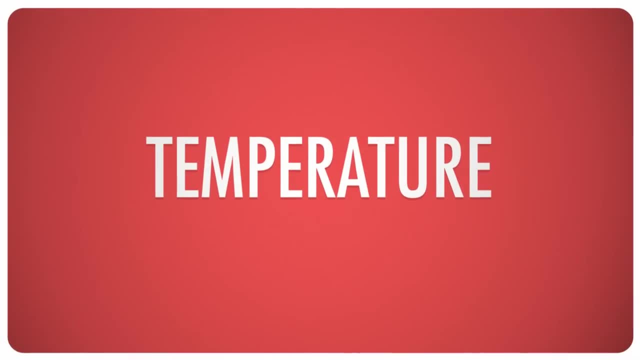 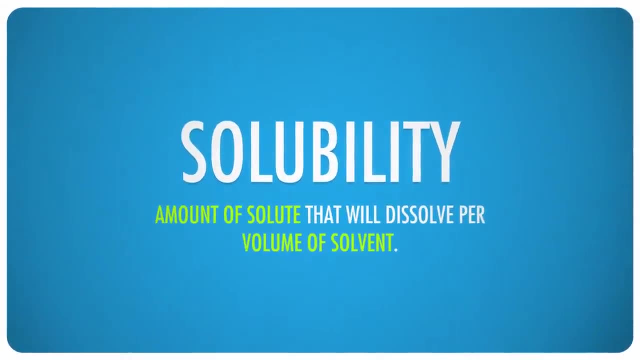 Finally, in addition to polarity and pressure, it's temperature that affects solubility in the most complicated and therefore interesting matter. When we're dealing with solid solutes and liquid solvents, their total solubility generally goes up as temperature increases. This is a fact that you already know, if you've ever 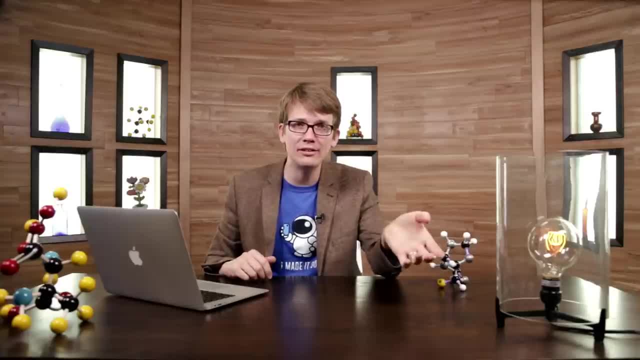 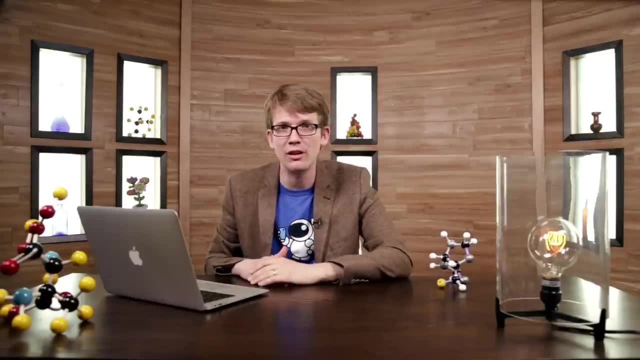 tried to put a bunch of sugar into your iced coffee. The solubility of gases, on the other hand, is the exact opposite, because colder molecules have less kinetic energy and are less likely to escape the surface of the liquid. So the upward pressure they exert is lower than it would be in a hot liquid. That's why it's safer and cleaner to open a can of soda pop when it's cold rather than when it's hot. While this phenomenon might result in a bit of a mess in your house, it's a much bigger. 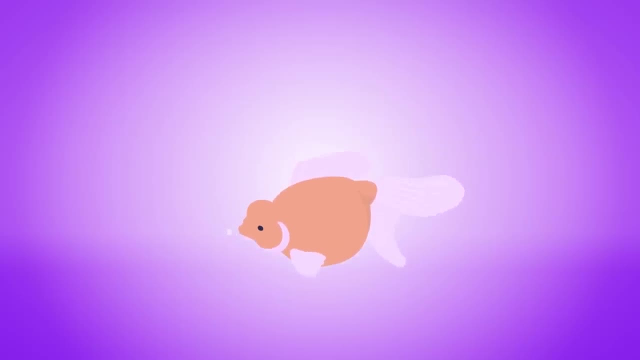 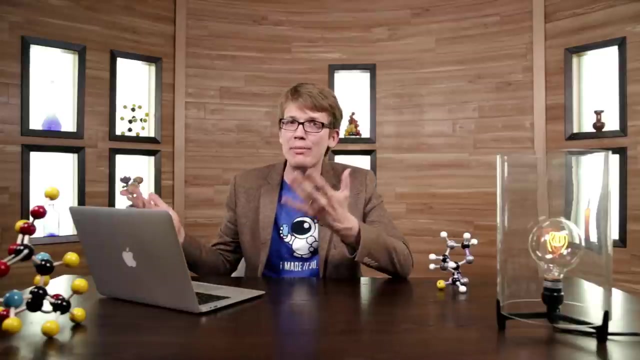 deal for fish who need oxygen dissolved in water to like breathe. At 4 degrees Celsius the solubility of oxygen in water is about double that of what it is at 25 degrees Celsius. Trout here in Montana are highly evolved to that nice oxygen-rich. 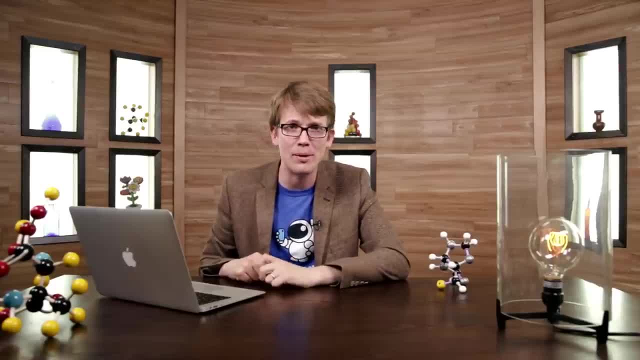 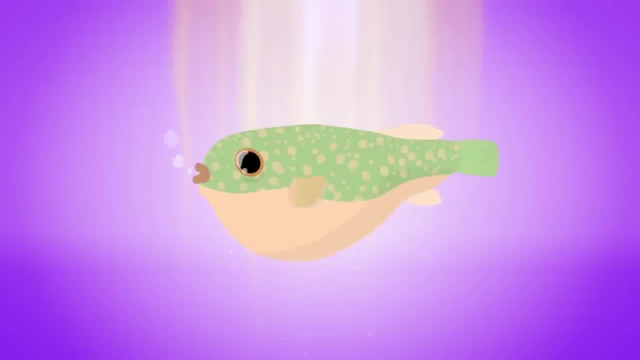 water, But summer heat waves can cause the amount of oxygen in the water to drop dramatically and cold-water fish can get pretty unhappy, Also a little dead. Fortunately for fugu it's a tropical fish, so it's perfectly evolved for 2020.. 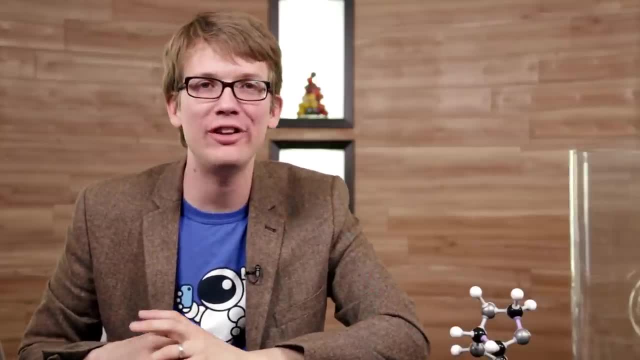 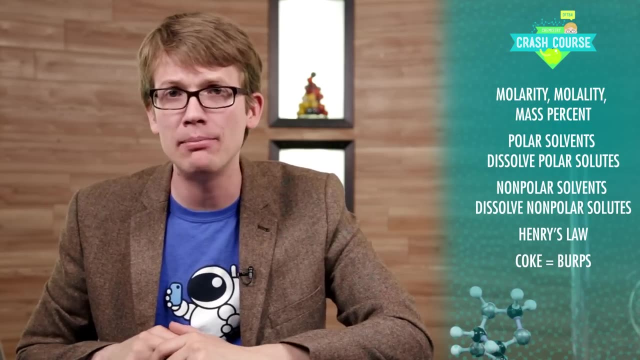 And unfortunately for all of us. that brings us to the end of this episode of Crash Course Chemistry. If you've been paying attention today, you learned that solutions can be described in terms of molarity. molality or mass percent, that polar solvents tend to dissolve polar